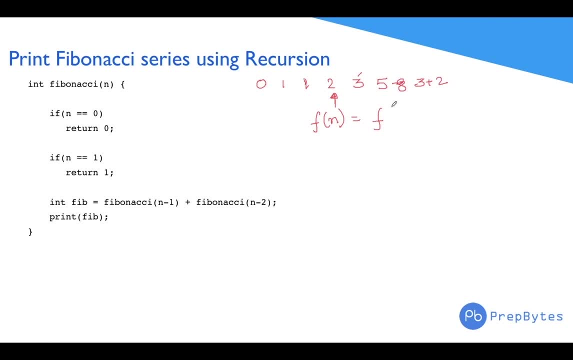 the value is equivalent to f of n minus one plus f of n minus two. So if we have to know that, let's say this is zeroth element. this is first, this is second, third, fourth, fifth, sixth. So if we have to know what is the sixth element, what do you? what is the value of sixth element in this Fibonacci? 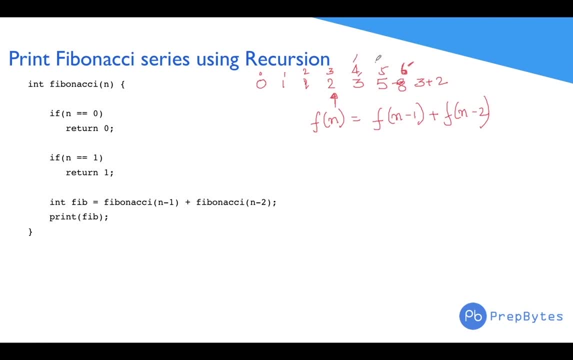 series. we need to know what is the value of fourth element and the fifth element, right And for fifth, we need to know what is the value of fourth element and the fifth element. So, if we have to, we need to know what is the value of fifth element and the fifth element. So, if we have to, 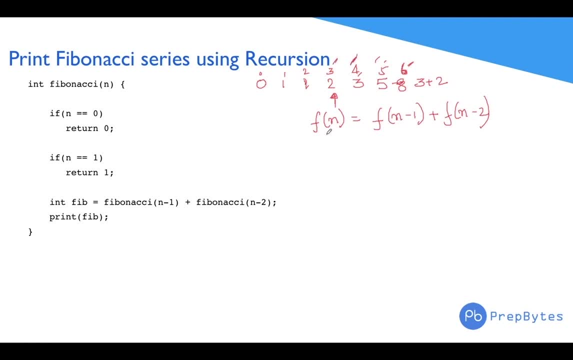 fourth and third right. So for any given number, Fibonacci, For any given number in a Fibonacci series is equal to f of n minus 1 plus f of n minus two. for n greater than 1.. For n equal to 1 it will be 1.. And for n equal to 0 it will be 0.. So now we have come up with the relation and these: 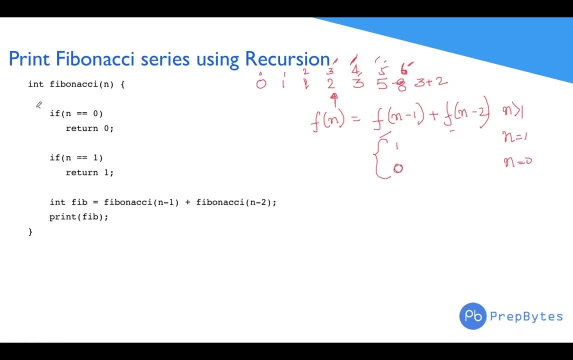 two will act as base conditions. So we have written the base conditions here. now we have written the function here. so Fibonacci is the function. it will accept a parameter, integer, parameter n, and it will return an integer. so what is this particular thing doing? so let's say I have to calculate that. what is the value? 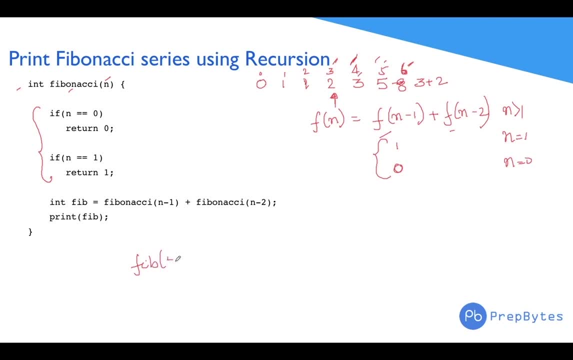 of fib 5. so for knowing what is the value of fib 5, we need to calculate fib 3 and fib 2, and for knowing the value of fib 3, we are calculating fib 2 and fib 1. so we are doing the same thing. we are breaking the problem into sub problems. 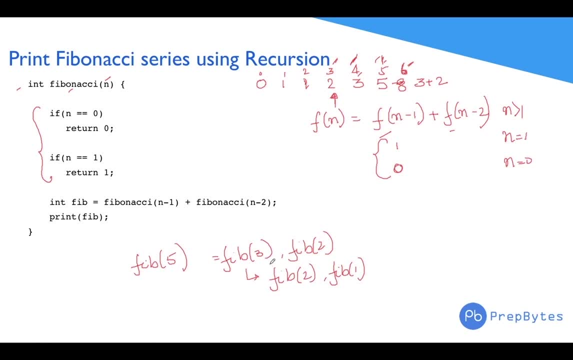 and we are doing the same thing, just changing the parameters. so this is where we use recursion, right? so we are doing the same thing, it's just that the parameters are getting changed. so now let's try to solve this using a recursion tree, using a tree. so let's say we have to print the series 3. 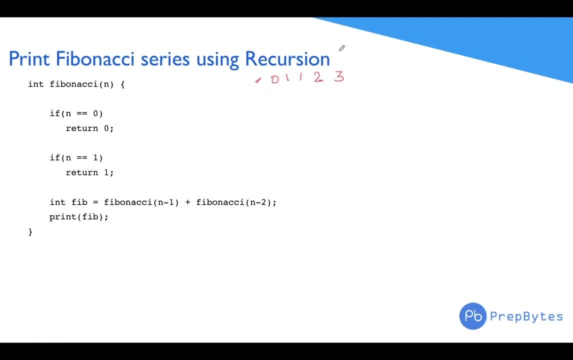 this particular series. now, to print these particular series, we need to know each value. so let's see how are we calculating each value and printing them. so let's say the program starts with fib 4. okay, so when n is equal to 4, fib 4. 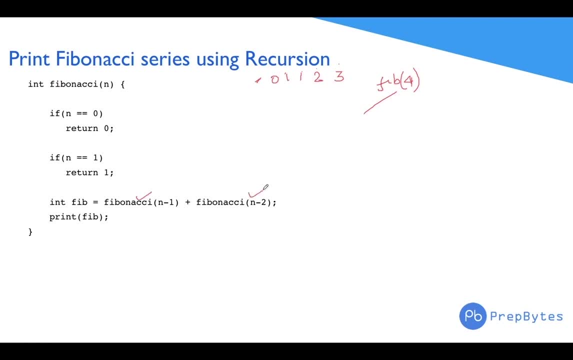 further calls fib 3 and fib 2. right fib 2 and fib 3, now fib 3. further calls fib 2 and fib 1. fib 2 further calls fib 1 and fib 0. now let's these. this is the tree that we make. let's see how. execution flows. so fib 4 calls fib 1 and fib 2, and fib 2 and fib 3 are equal to 3. fib 3 and fib 2 and fib 1 are equal to 3. now fib 3 and fib 2 are equal to 3, now fib 3 is. 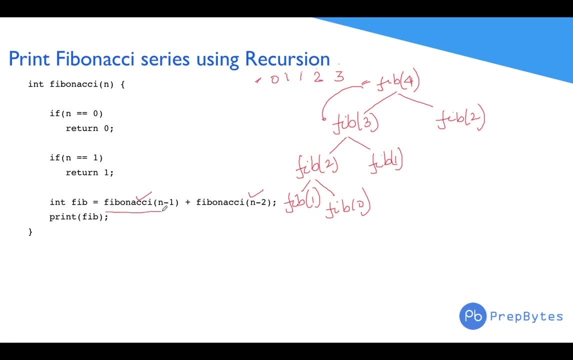 calls fib 3 first. right, so fib 3 is called from here. and as soon as fib 3 gets called, we go back to this particular place. we go back to this particular place, right. so now our n becomes 3. we check these conditions. they are not true. now we call fib 2 again. fib 2 is called from here. 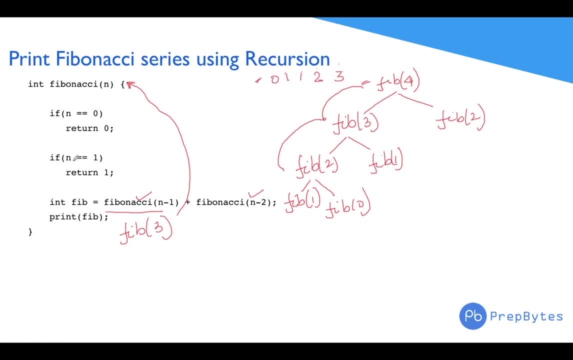 we come back here we check if these conditions are true. no, we call fib 1 and as soon as we call fib 1. so I'll write it down here also. okay, so it will make us easier to understand. so fib 4 calls fib 3 and fib 2. fib 3 calls fib 2 and fib 1. fib 2 calls fib 1 plus. fib 3 calls fib 2 and fib 1. 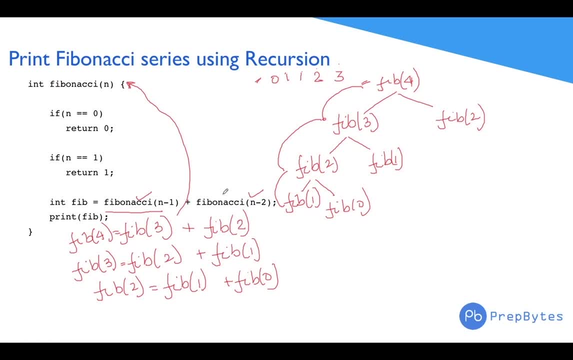 0. so this is how the calls are being made. so now, first this particular call is being made and only when this particular call has given me the answer, we go to this particular call. I'll make you understand. so, coming back here, we have fib 4, fib 3, fib 2, fib 1. now we are here right now in the 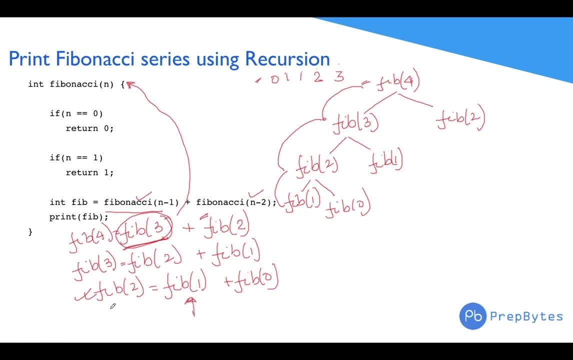 tree, fib 2 called fib 1, right, so fib 2 called fib 1. fib 1 gives us the value of 1 for n equal to equal to 1. so this particular function gives returns the value of 1 to fib 2. so here we get the value. 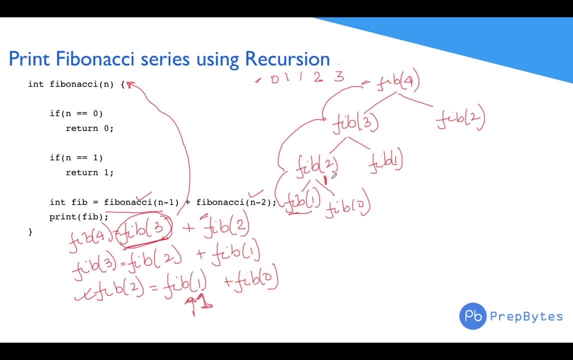 1. so here for fib 2 gets the value 1 from fib 1 plus. now what happens when fib 1 returns the value? now fib 2 gets called. okay, now fib 2 gets called. so this is how the execution goes. it starts from the left and then it goes to the right. so this is how the execution goes. so now fib 2: 0 is. 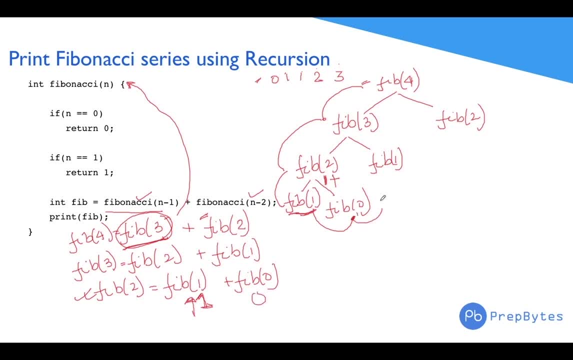 called fib 0 returns 0. so fib 0 returns 0 to fib 2, since fib 2 was the one which called fib 0. so now we get fib 2 as 1 plus 1, equivalent to sorry, 1 plus 0 equivalent to 1. now this fib 2 will return. 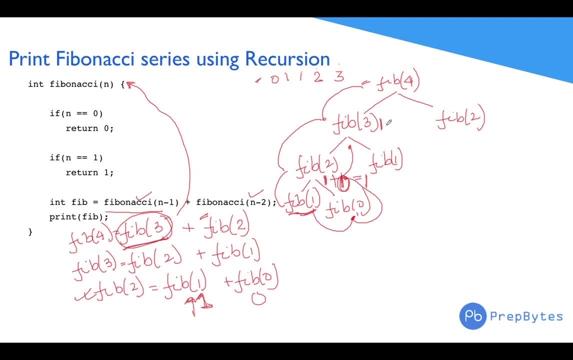 this 1 to fib 3, so this fib 2 returns 1. now, as soon as we get 1 here now, this fib 1 gets called. this fib 1 gets called. now. this fib 1 also returns 1 to fib 3, so fib 3 now gets the value as 1 plus. 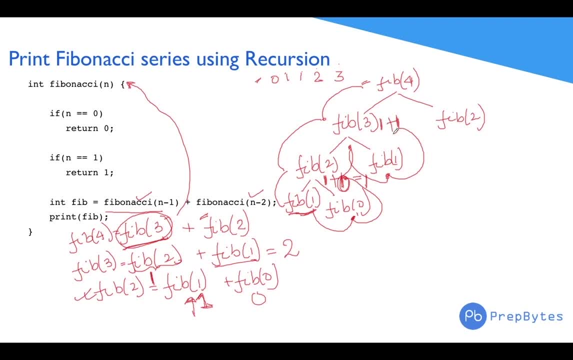 1 equivalent to 2. so this fib 3 returns 2 to fib 4. so this fib n minus 1 execution has been done for fib 4. this execution has been done and as soon as this execution finishes, the control comes back here. now we come here. we come to fib 2. now, again from here, fib 2 returns 1 to fib 3, so fib 2 returns. 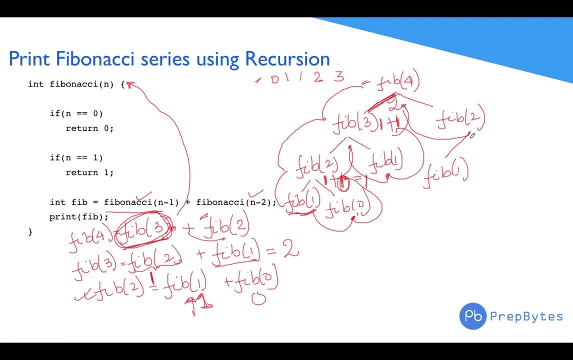 fib 2 calls fib 1 and fib 0. fib 1 returns 1 to fib 2, fib 0 returns 0 to fib 2. fib 2 get the values as 1 and fib 2 now returns this 1 to fib 4. so the value of fib 4 gets 2 plus 1, equivalent to 3. the 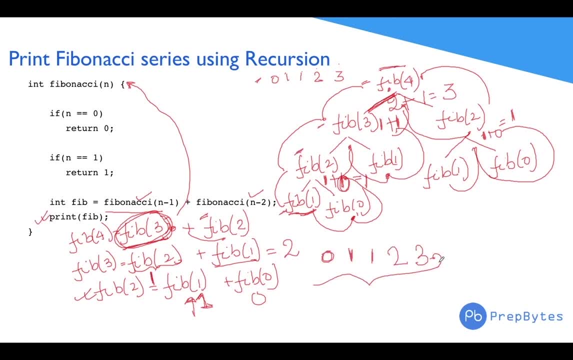 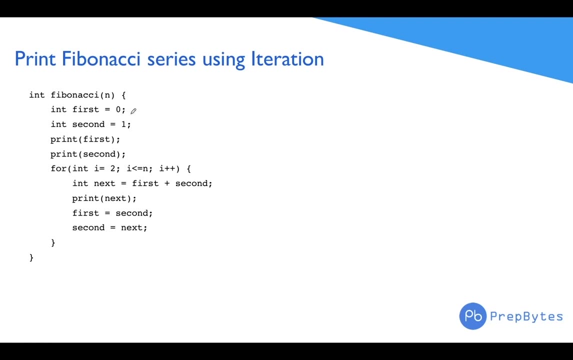 value of fib 4. so this is how we did it using recursion. so this is how we did it using recursion. now we can do the same thing using iteration as well. let's see the code for iteration. now let's see how we can print fib series using iteration. so we have first equal to 0, first, and second gets. 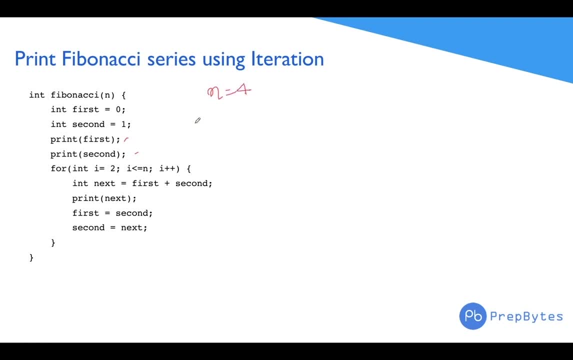 printed. so let's say we have to print till n is equal to 4. okay, so first and 0. second gets printed 0 and 1, so then we have print. then we run a loop from 2 to n, which is 2 to 4, so for i equal to 2. 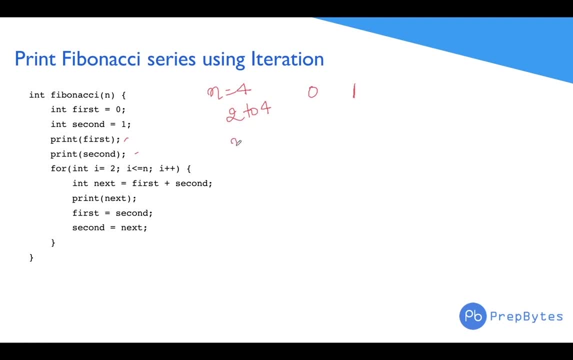 we get next equal to 1st plus second. so next gets the value as 0 plus 1. next gets printed: first becomes second. so now my first becomes 1 and my second becomes 1 as well. okay, so every time the previous two elements are getting updated. now we have i equal to 3, for i equal to. 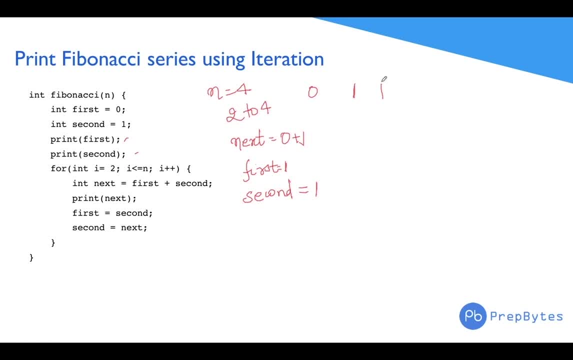 3 for i equal to 3. this is for my first and second, and then this is my second, and then this is again. my next is first plus second, which is 1 plus 1, 2, so 2 gets printed. now I again update my first. now my first becomes this and my second becomes this: 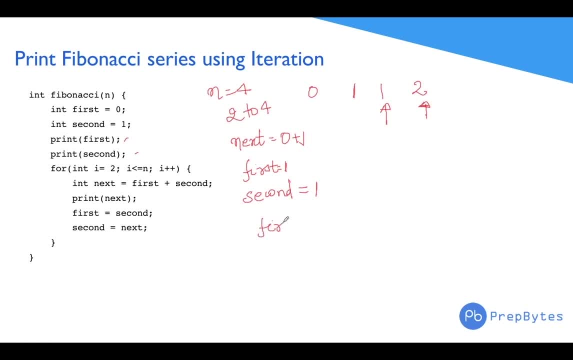 so I'll update my first to 1 and my second to 2. now again, my i becomes 4. now and we have next equal to first plus second, which is 3. 3 gets printed. and then again we do this: our first become 2 and our second becomes 3. now we again. 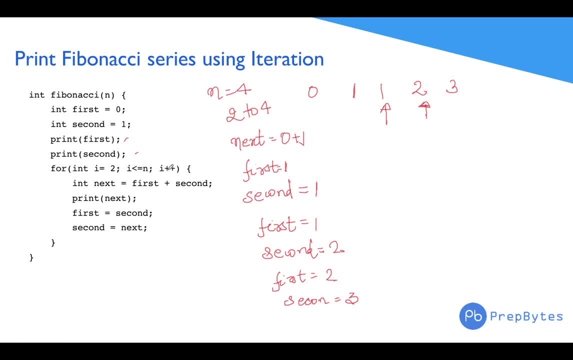 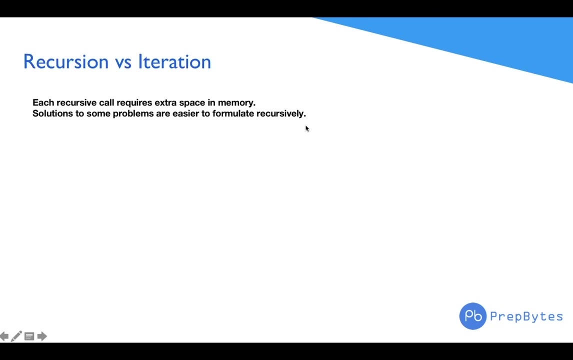 increment our i, but since our i is now greater than n, the loop is broken. so we can print Fibonacci series both using iteration and recursion. so let's see what are the differences between the two, differences between iteration and recursion. so, though, there are many differences, and first, so let's say what is the agenda of knowing this, you might 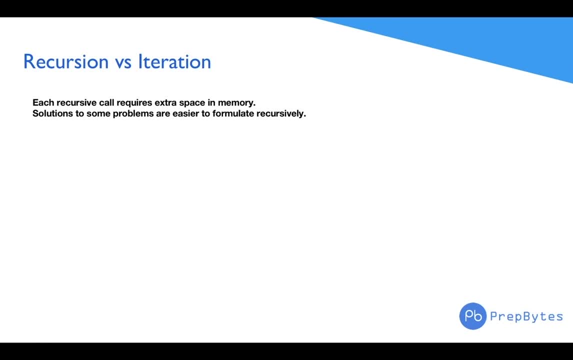 be knowing this because you have to write it in exam, or there might be a reason that you want to know this so that you can write correct code. you can write a recursion where it's needed and iteration where it's needed. so few very common differences, I'll tell you. is that so like we have? 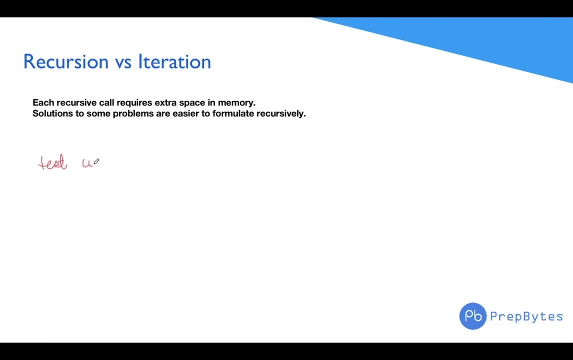 test conditions in loops. we have base conditions in recursion right. so your loop breaks when the test condition is false and your recursion terminates when your base condition is true. number one. number two: that if you do not put this test condition, you will get into an infinite loop. 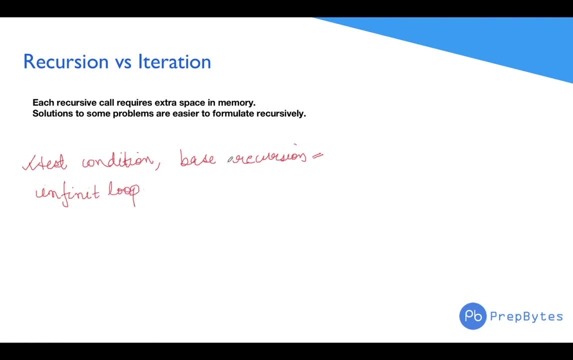 and in case of recursion, if you do not put the base condition, you will get stack overflow error. so the recursive call will be made again and again and that will continue until that stack is full and you get stack overflow. so now the question is: why is that? this is getting into an infinite loop. there is no out of. 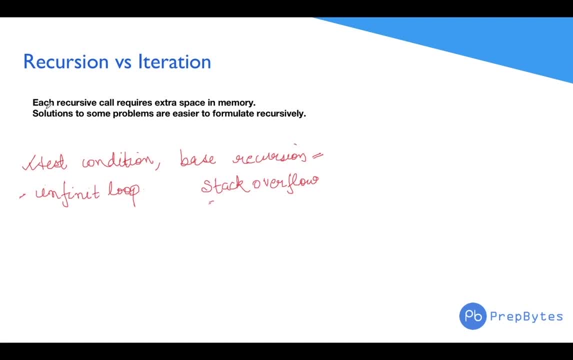 memory thing here. but we are getting it here because in order to get that stack recursive call requires extra space of memory. so, as we discussed that, recursive calls are stored in stack, so each recursive calls make a copy of method, of the variables, of the parameters. so we need extra space. so whenever there is a 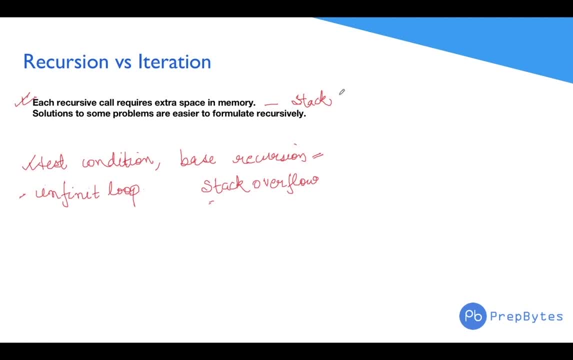 code that can be written very easily using iteration. you should prefer using iteration, but there are some solutions to some problems which are not very easy or very straightforward using iteration. so as, as we saw that there are branches right, so there must be that there are several possibilities for our 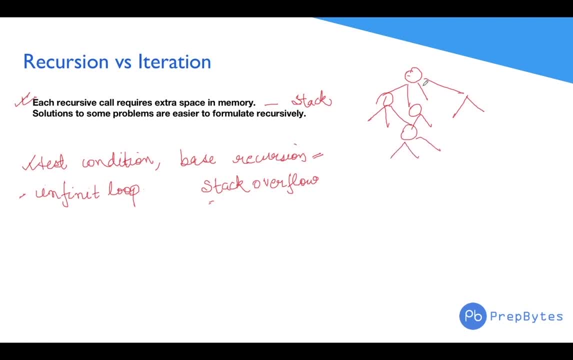 solution. so in this case, especially when there, when we have lots of possibilities, we cannot track each possibility using iteration, but it's very, it becomes very easy to take these kind of things using recursion. so when you have a problem statement which has lots of possibilities and it's difficult to track that using iteration, go for recursion and if you 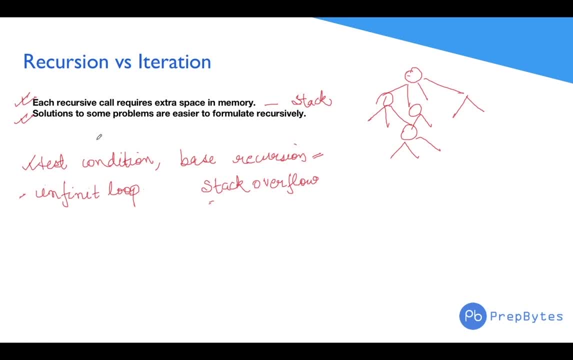 have a problem statement which is: which is very simple and can be done using both, and can be easily done using both of this. you should use iteration because iteration don't require any extra memory, whereas recursion does. so that was about recursion and iteration. we will keep on.